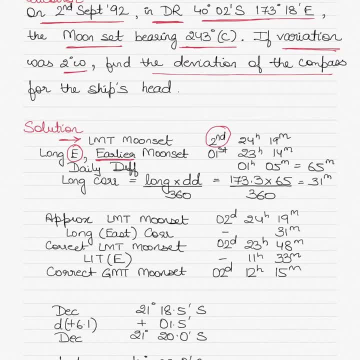 because we have the east longitude. So whenever it's the east longitude you find out the LMT moon set for the day in question as well as for the earlier day. If it's west longitude, you would find out for the day in question and the next day. So it would have. 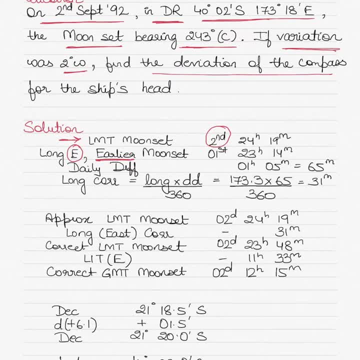 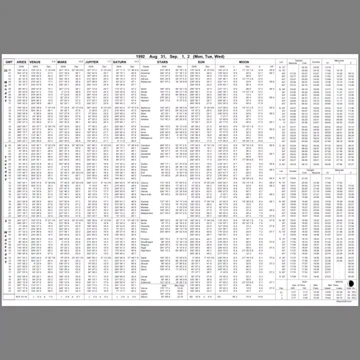 been 3rd if it was west longitude, Because it's east longitude. you will be finding it out for the day in question and the earlier day. So what we do is we go into the nautical almanac and then you can see here. I'll show you where to do that. So this is the moon set time given here. You see here. 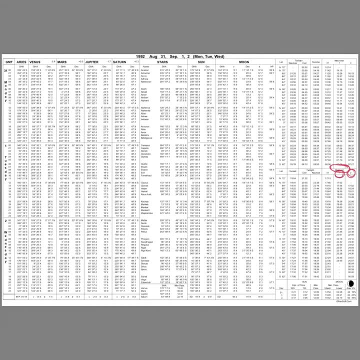 this is for the 2nd of September. this is for the 1st of September. Now you have to go and find it out for the particular latitude. So latitude is about 40 degrees or south. Alright, so south is here and 40 degrees is somewhere here. So you can see, the date in question is 2nd of September. The latitude: 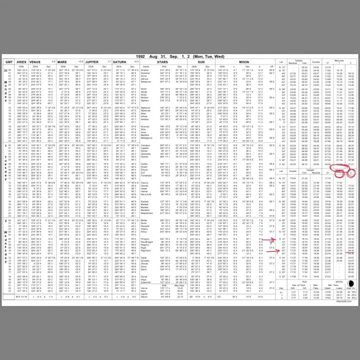 is 40 degrees south. The days are 2nd of September, moon set, and 1st of September, moon set, 24, 19 and 23, 14.. So when we say 24, 19, of course we mean after midnight 0019.. But we write as 24, 19 sometimes. 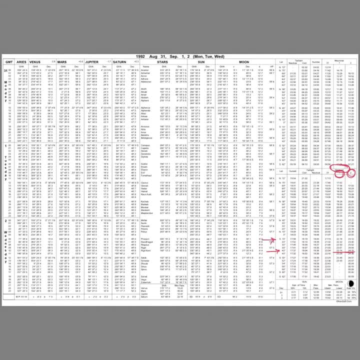 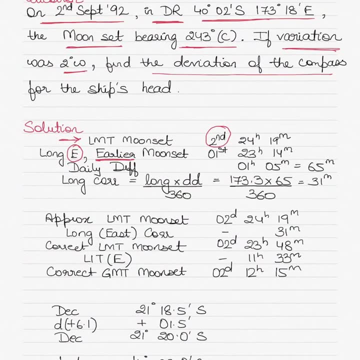 to make the mathematics easier. Alright, so pause the video here. see how I got the times from, and once you understand, only then you move on to the solution For me. I'll keep going. So I have got both the times here, and what I'll do is I'll find out the difference between the two, So find out the. 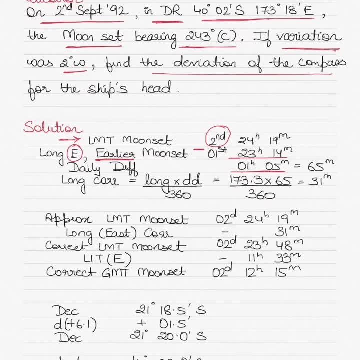 difference between the two. in this case, you get as 1 hour 5 minutes, which is equal to 65 minutes, So 1 hour 5 minutes is 65 minutes. Why? Because 1 hour 5 minutes is 65 minutes, So 1 hour 5 minutes is 65 minutes. 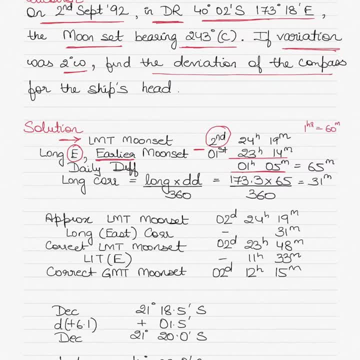 Because 1 hour equals to 60 minutes, And then, of course, you add the 5 minutes and you get 65 minutes. Now, using this time, you find out the longitude correction. How do you do that? You convert longitude into decimals first, Alright, and multiply it with the daily difference, dividing. 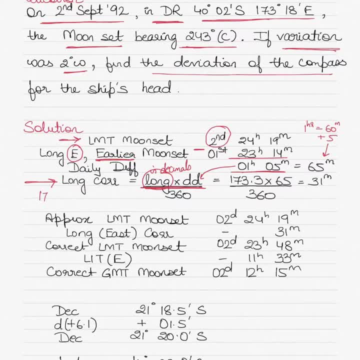 it by 360.. So how do you convert 173 degrees, 18 minutes, into decimals? Just divide 18 by 60. When you divide 18 by 60, you get what? 0.3.. So your longitude would be 173.3.. That is how you convert the longitude into. 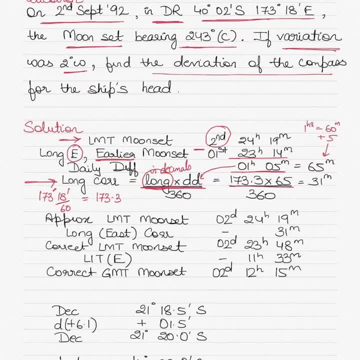 decimals, Then multiply it by the daily difference, which is 65 minutes, and divide it by 360. you get 31 minutes. When you get 31 minutes and it's longitude, you will add a minus to it. This is a negative 31 minutes. If it was West, you would have kept it positive. So again you come back to 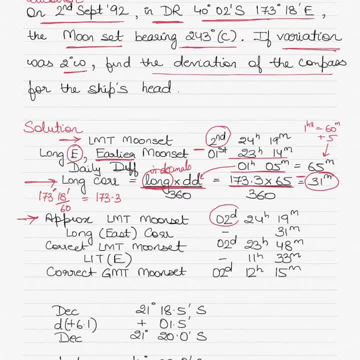 approximate local mean time moon set for 2nd of September 2419, apply your correction to it, The correction that you calculated, because it's East longitude. you will subtract it. You get your correct local mean time of the moon set. 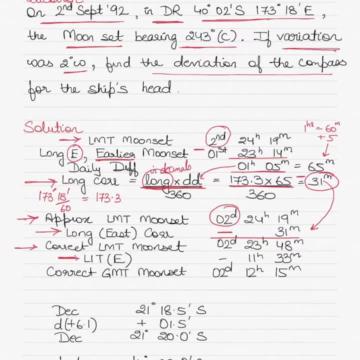 Do that? you apply your LIT, or longitude in time. Your longitude in time is found out by dividing longitude by 15.. So divide 173 degrees, 18 minutes by 15. And you will get 11 hours 33 minutes. Whenever it's East longitude. 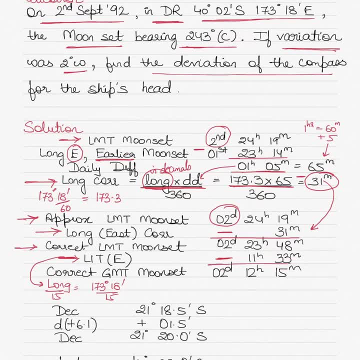 from LMT. because longitude East GMT is least. LMT is more than GMT. longitude West GMT is the best. GMT is more than LMT. so you subtract it from the local mean time of the 2nd of September and what you get is the GMT time for the 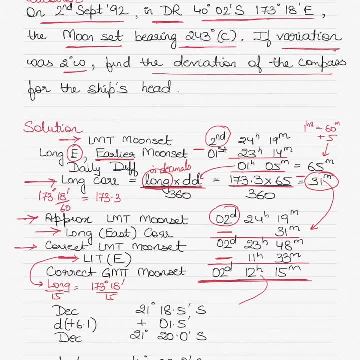 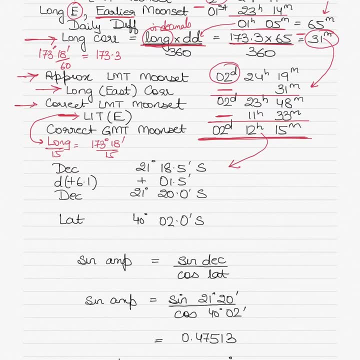 2nd of September, 12 hours 15 minutes. this is the time that you will use to find out the declination of the moon. all right, so find out the declination of the moon for 12 hours on 2nd of September, then find out the D value here and then. 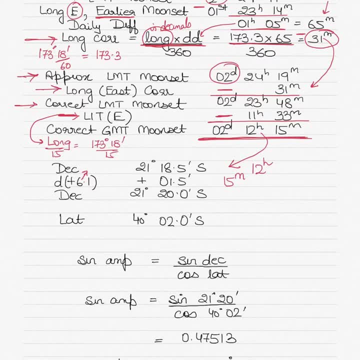 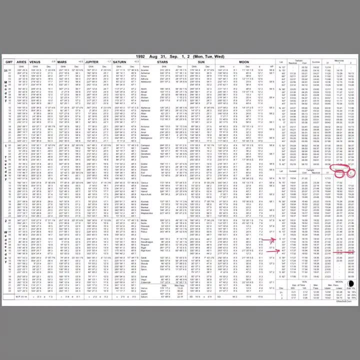 go into the increments page for 15 minutes and I'll show you where at the rest. so we'll go into the 2nd of September for 12 hours. I'll find out the declination value and the D value. so 2nd of September is here. 12 hours is here my. 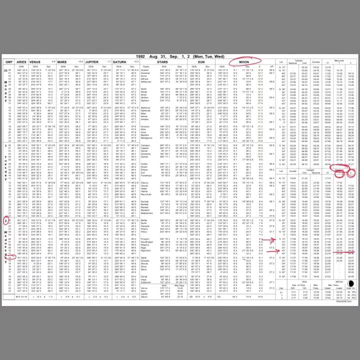 moon is here, so my declination will be 21 degrees 18.5 Celsius. my D value is 6.1 and because my declination is increasing from 12 hours to 13 hours, I will be adding the D correction that I will find out later. 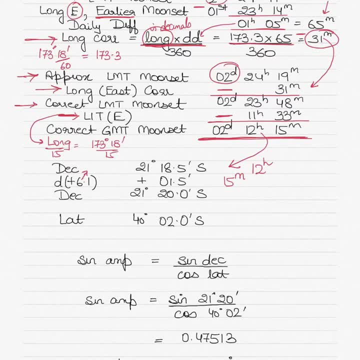 all right, so you could have paused that video there itself and you had seen whether we know how I got the values of declination and D value. so I've got these values and now I will be using the D value of 6.1, going into the 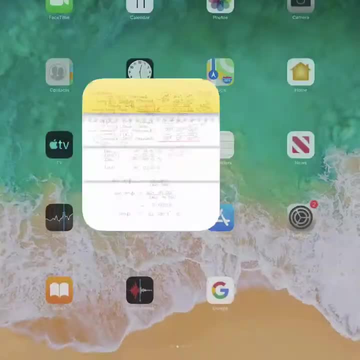 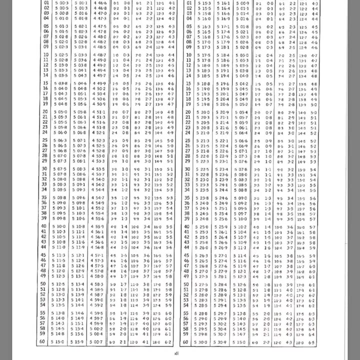 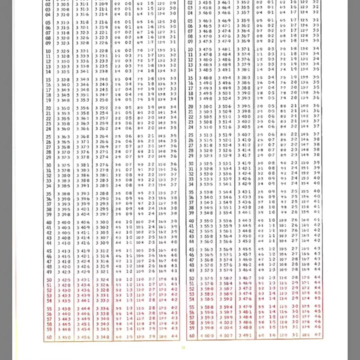 increments page for 15 minutes to find out the D correction value. so I go back into the increments page, the nautical almanac, for 15 minutes. so you can see that D is here and we have an inscrement of 12 hours total. that's it. so it will be 6.1 which will be here somewhere. that's right, it's here. so 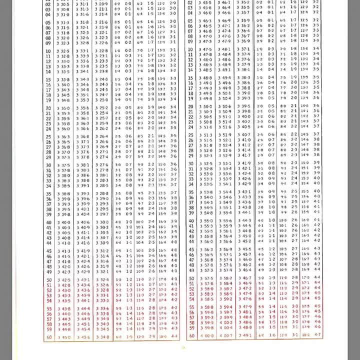 what I'll do is this is 50 minutes. my D value is the one in this column here, and my D value is 6.1. it will be somewhere here, all right, so it's here, and the correction value is 1.6. this is the correction I will add because of my 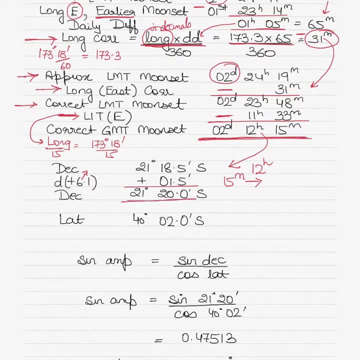 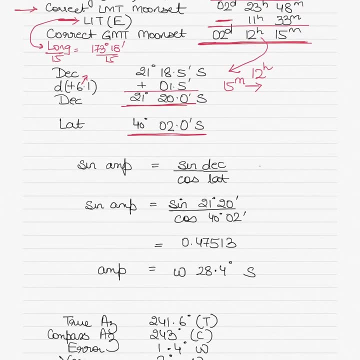 declination was increasing from 12 hours to 13.0, it plus 1.5. I have got my declination. my dL latitude is given to me in the question already. then it is simply a matter of putting it in the formula: sin amplitude equals sin declination. 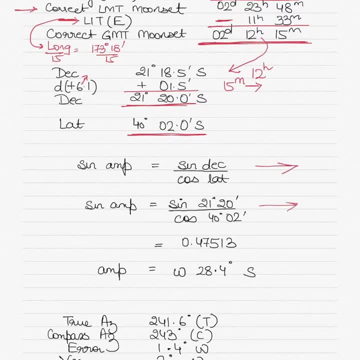 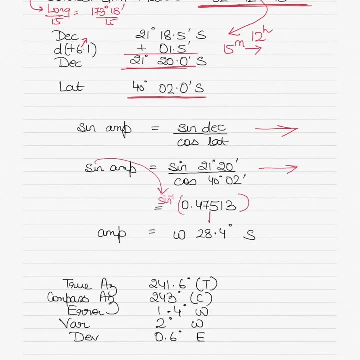 divided by cos of latitude. put the figures in, get the value. can put sin here. you get sin inverse of this value here, which will give you the amplitude value of 28.4 degrees. now, 28.4 degrees, I have put west and south here. why? 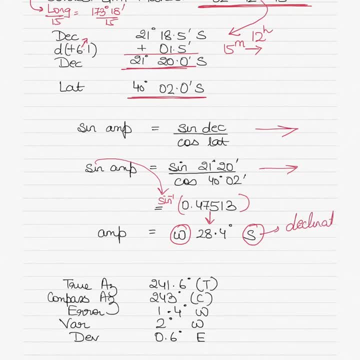 this south comes from declination. alright, the west here comes because the moon is setting. the moon is setting, celestial body is setting its setting on the west. so we put west. if it was rising, i would put east. south is declination. always put weather is rising and setting first. 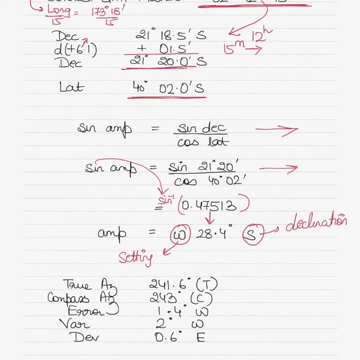 and then put the declination. don't do it the other way around. all the other cases you put south or north first, then you put east, west, but in this case you put south and then you put west, then you put east, but in this case 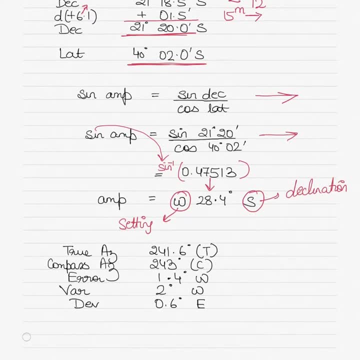 case you will be doing the opposite. you will be putting whether it's rising or setting first, and then you will be putting the declination so it will make it west, south or east south or east north or west north. all right now, west 28.4 south. what does that mean? that means 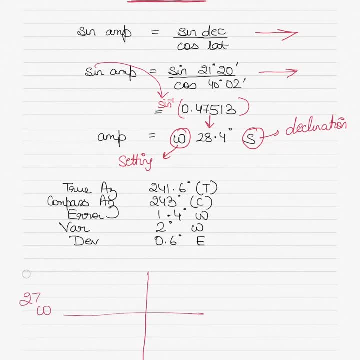 west is here, which is 270, and south is here, which is 180, going down: 28.4 from west. 28.4 from west, that means 270 minus 28.4. 270 minus 28.4 is 241.6. that's how i got my true azimuth. 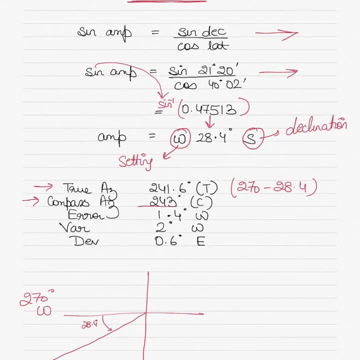 the compass azimuth is given to you in the question 243 degrees. compass is more compass, best error is west. so 243 minus 241.6 will give you your compass error. and because compass is more error is west, then the variation is given to you in the question two degrees west. 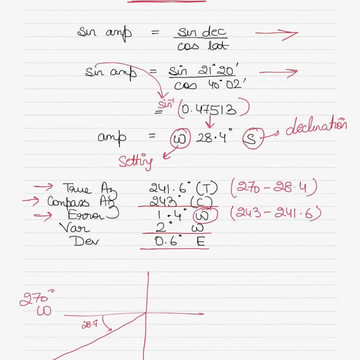 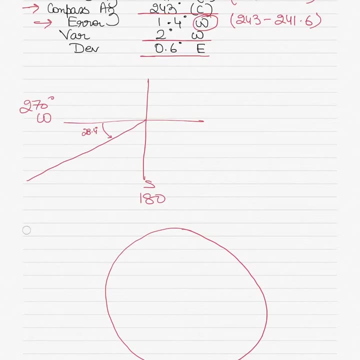 so your deviation will be 0.6 degrees east. all right, how is that? let's look at this conceptually. so draw a circle here. put your true bearing as 241.6 is your true. your compass is 243. it will be west of true 243. so your error will be automatically west by 1.4 degrees west. 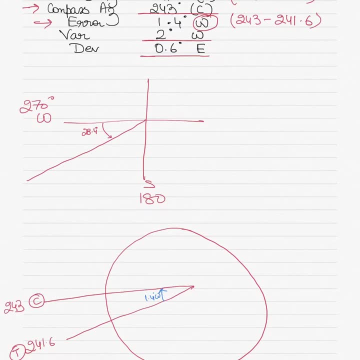 then you have to put your variation. your variation is what? two degrees west? variation is the angle between true and magnetic, where magnetic is to the west of true, so your magnetic will be here. this angle is your variation, and then variation of two degrees west, so two degrees will be more than that. right, sorry, my apologies, so i'll delete it. sometimes i'm 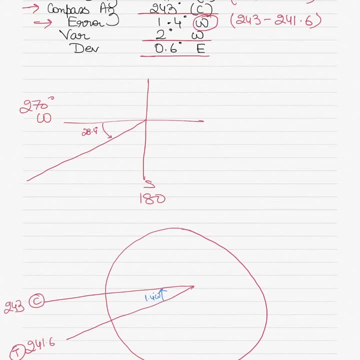 allowed to make errors. come on, guys, all right. so variation is between true and magnetic, where magnetic is to the west of true. so it will be 243.6 somewhere here. that's right, all right, yeah, minute, okay. so this red is two degrees west, all right, and that's why your 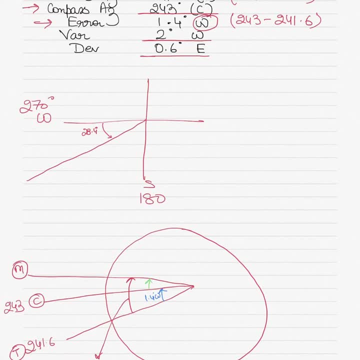 deviation will be this angle here, this small angle here. all right, and because your compass is to the east of magnetic, so compass is to the east of magnetic, so this value is the deviation, which is 0.6 degrees east. okay, so that's how i have calculated.